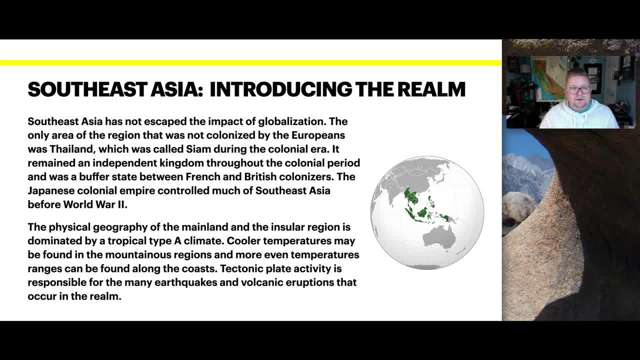 in this presentation. Now, Southeast Asia has not escaped the impact of globalization. The only area of region that was not colonized by Europeans was Thailand, which at that point was called Siam. It remained an independent kingdom throughout the colonial period and was a buffer state between French and British colonizers. 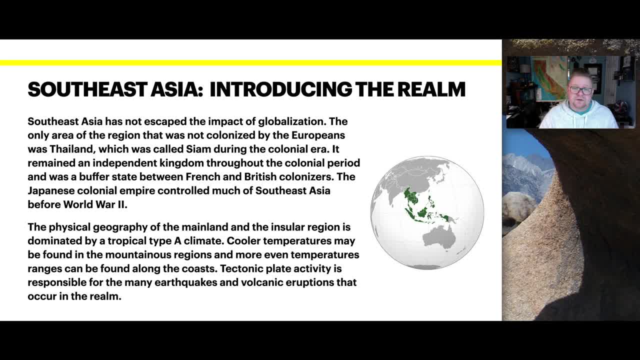 The Japanese colonial empire controlled much of the southeast before World War II. The physical geography of the mainland and the insular region is dominated by tropical A-climates. Cooler temperatures may be found in the mountainous regions and even more temperate ranges can be found. 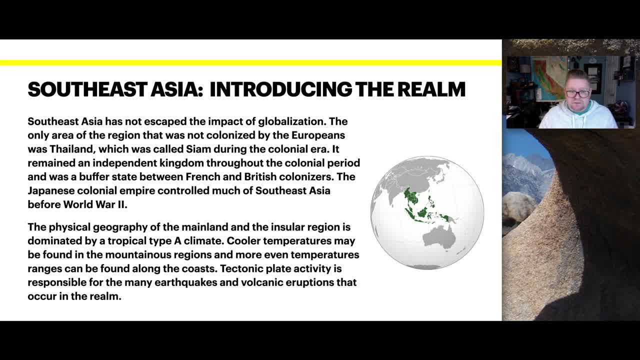 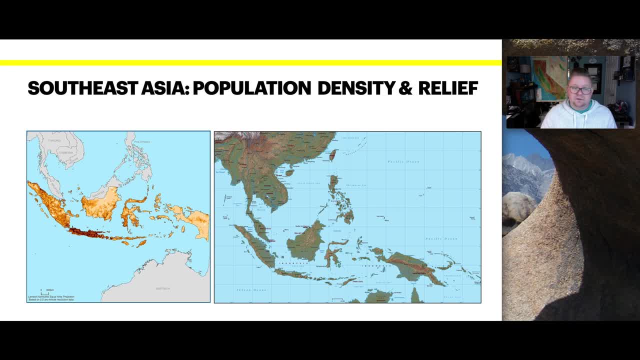 along the coast. A tectonic planet activity is responsible for many of the earthquakes and the volcanic eruptions that occur within the realm. So, again going with our classic dot density map and then also looking at a raged relief, I couldn't find a really good dot density that had both mainland and the insular islands, but nonetheless we can really see. 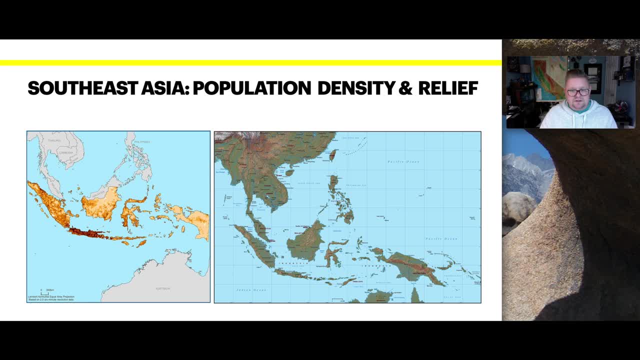 the patterns. So we certainly know that a majority of these environments, as we'll continue to speak to, are volcanic based. And, that being said, you know, since we've got all these different accumulations of islands, we'll learn a little bit about the resources that are prominent in those landscapes. 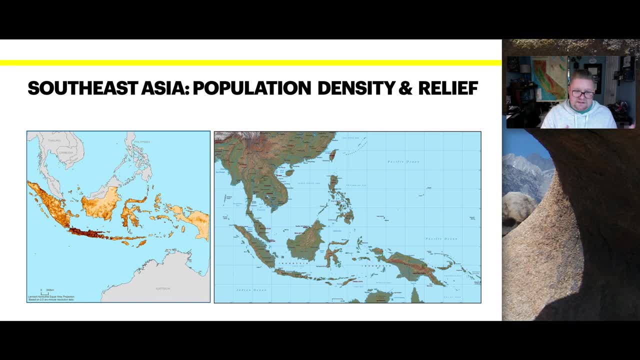 but again, we can certainly see that there is population densities farther on the western ridge And you know, when we start discussing about things like that in the text and throughout the course, think about why. You know, when it comes to trade, when it comes to transport, when it comes to 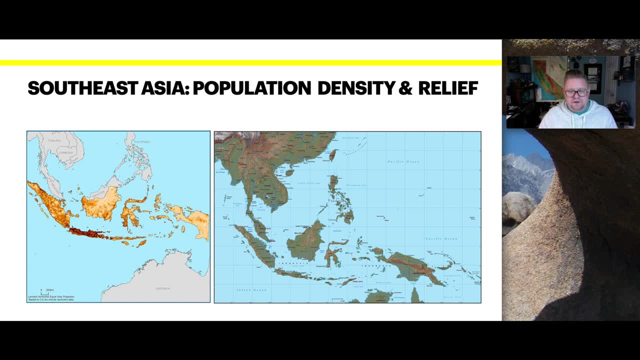 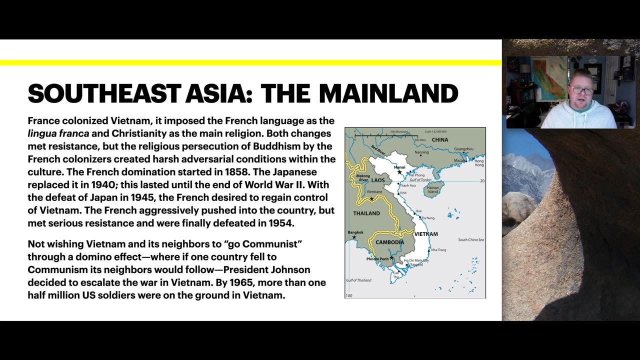 export of goods and things like that. those are really great things to take into consideration. But again, do we see a relationship with topography And the land landscape when looking at population density? so let's talk about the mainland first. so now France colonized Vietnam. it imposed the French language as the 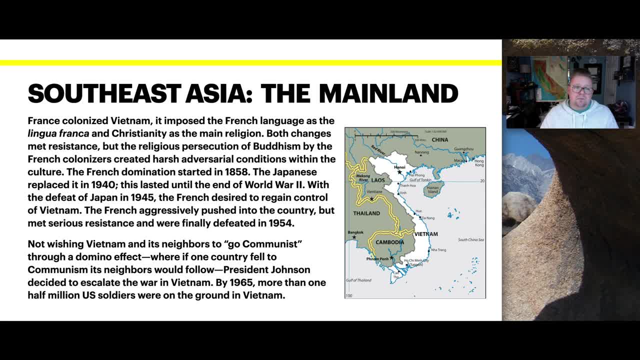 lingua franca and Christianity as the main religion. both changes met resistance, but religious persecution of Buddhism by the French colonizers created harsh adversarial conditions within the culture. the French who dominated. a domination started in 1858. the Japanese replaced it in 1940. in this 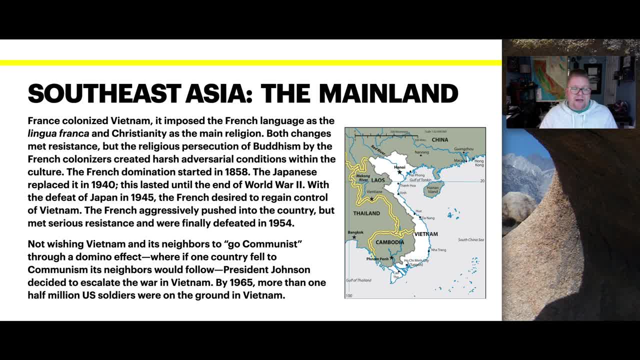 lasts until the end of World War two. with the defeat of Japan in 1945, the French desire to regain control of Vietnam. the French aggressively pushed into the country but met serious resistance and were finally defeated in 1954. now not wishing Vietnam and its neighbors to go communist through a 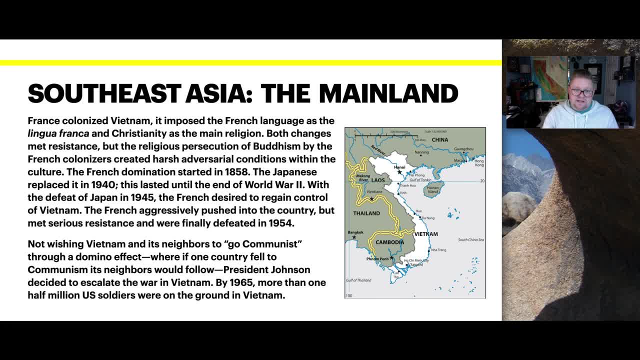 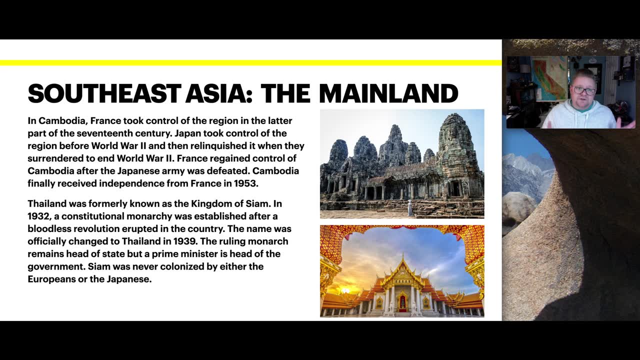 domino effect, where if one country fell into communism, its neighborhoods would follow. President Johnson decided to escalate the war in Vietnam, and by 1965 more than one and a half million US soldiers were in the ground in Vietnam. you now in Cambodia. France took control of the region in the latter part of the 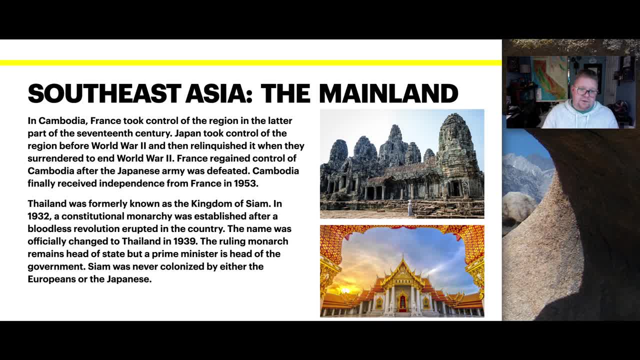 17th century. Japan took control right before World War two and then relinquished it when they surrendered at the end of World War two. France regained control of Cambodia after Japanese army was defeated and Cambodia finally received independence by France in 53. and what I did here is I wanted to 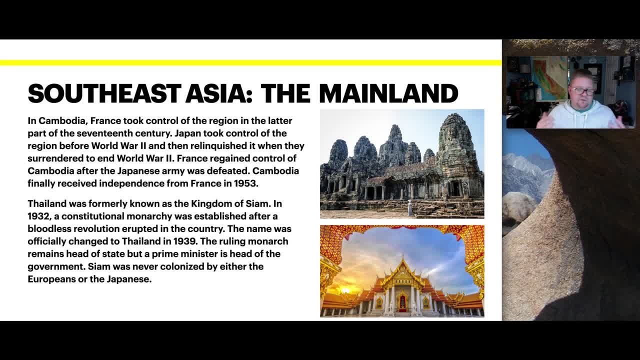 select two really interesting images, one from Cambodia and one from Thailand, and these are both of the temples of that realm and I just thought that was really interesting. when looking at that, you know and you know I don't, I guess when I look at architecture and stuff like this, you know I'm looking at the cultural. 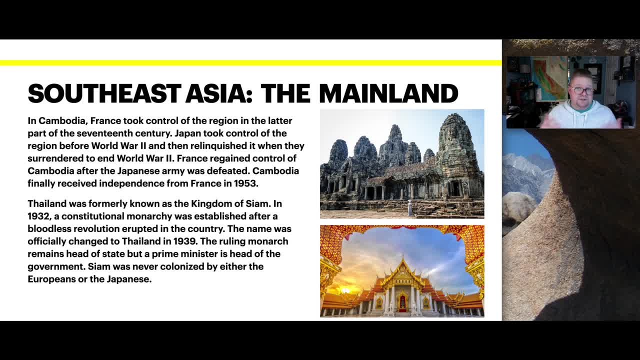 perspective, the time, the air in which would have been built, and also just think about the economics. so, moving forward, Thailand was formerly known as the Kingdom of Siam. in 1932, a constitutional monarchy was established after a bloodless revolution erupted in the country. the name was officially changed to Thailand in 1932. 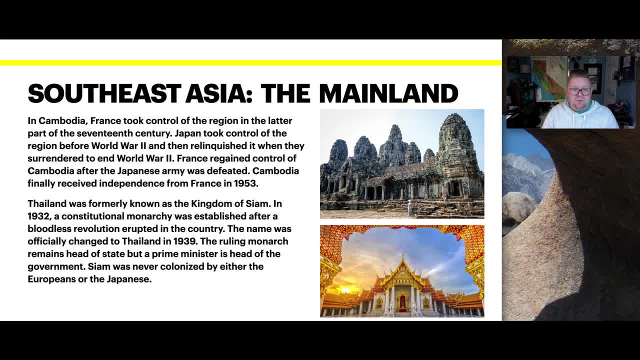 the name was officially changed to Thailand in 1932. the name was officially changed to Thailand in 1932. in 1939, the ruling Monarch remains head of state, but a prime minister is head of the government. Siam was never colonized by either the Europeans or Japanese. 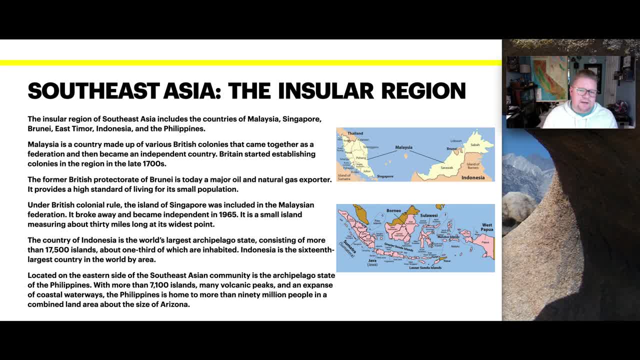 now introducing the insular region a little bit different in the mainland, because now we're looking specifically at these larger islands which I mentioned before were really established because of its volcanics. so the insular region of Southeast Asia includes countries of Malaysia, Singapore, Brunei, East Timor, Indonesia and the Philippines. now Malaysia is a country made up of various British 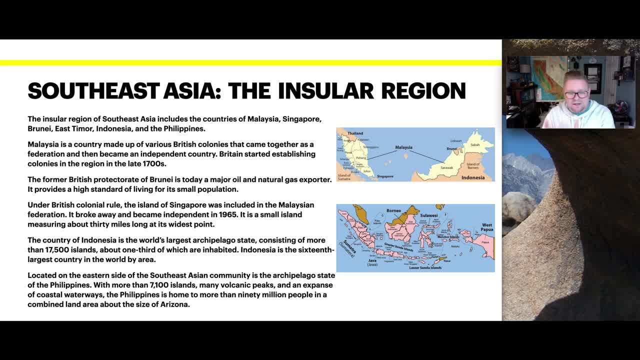 colonies that came together as a Federation and then became an independent country, Britain started establishing colonies. this region the late 1700s, the former British protectorate of Brunei, is today a major oil and natural gas exporter. it provides a high standard of living for its very small 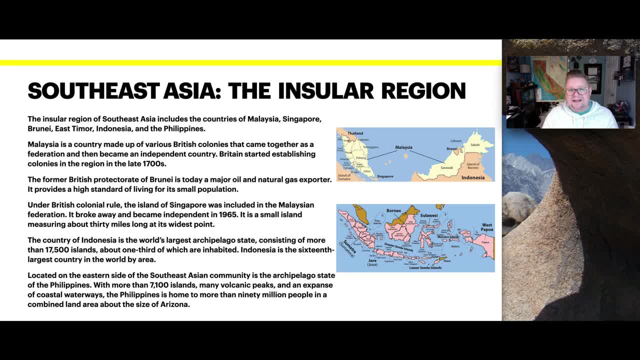 population. under British colonial rule, the island of Singapore was included in the Malaysian Federation. it broke away and became independent in 1965.. it is a small island, measuring only 30 miles long at its widest point. the country of Indonesia is the world's largest archipelagic State, consisting of more than 17 500. 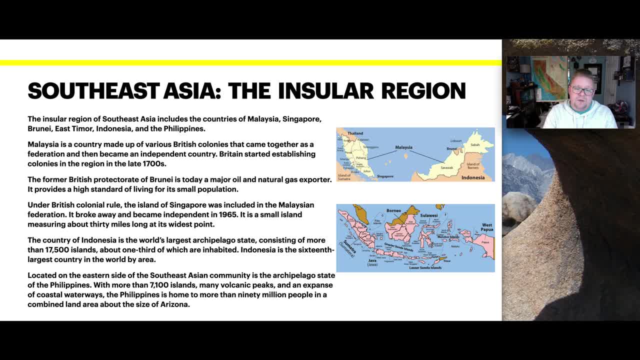 Islands about, of which one-third are inhabited. Indonesia is the 16th largest country in the world by area. now locate on the eastern side of the Southeast Asian Community is the state of the Philippines. with more than seven thousand one hundred islands, many of which are volcanic Peaks and an expanse and coastal waterways, the Philippines is 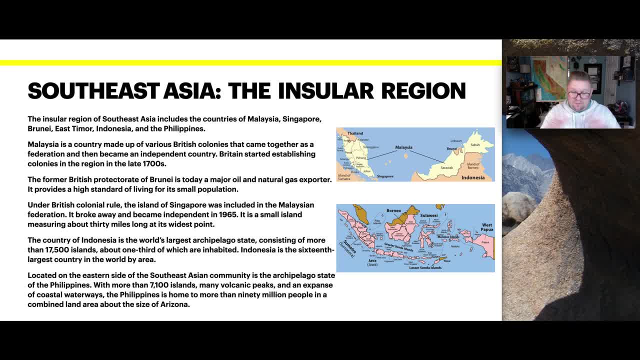 home to more than 90 million people in a component, in a combined land area equivalent to that of Arizona in the United States. so again, when we started speaking earlier on in this presentation, looking at locations, exports, transportation, where are people living? where does? where are those roots? 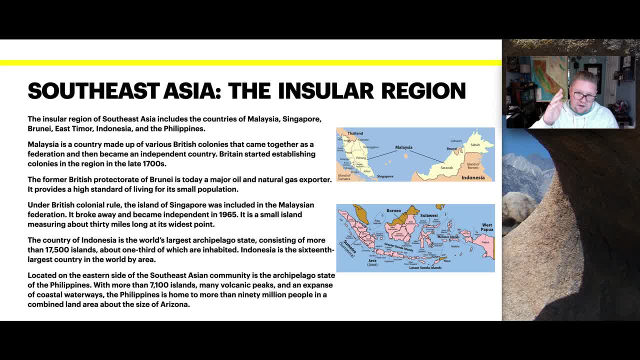 in play. also, you know just when you think about uh, more more recently, you know what's really kind of picking up in this area. aside from, you know natural exports of oil and gas technology, but also tourism, eco tourism is really starting to pick up in these areas, specifically in Thailand, and perhaps you've seen on the Travel Channel some of 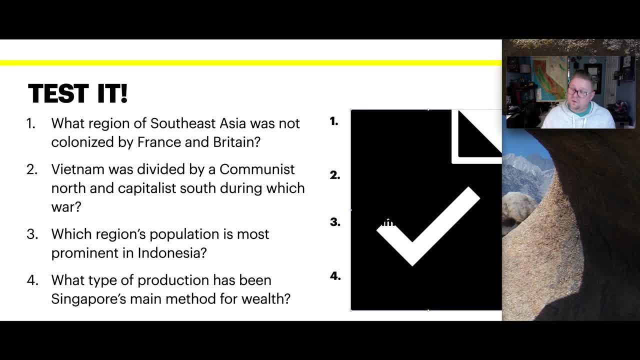 those locations which people like to travel to. all right, in our final slide, let's test it again. I gave you four questions that deal with not just the presentation but the reading within the course, and you will see these questions on your exam. so let's get going. question one: what region? 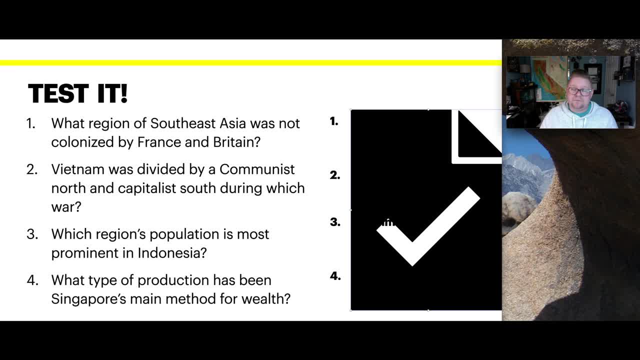 Southeast Asia was not colonized by France and Britain. Question number two: Vietnam was divided by a communist north and capitalist south during which war? Question three: which region's population is the most prominent in Indonesia? Question four: what type of production has been Singapore's main method of wealth?